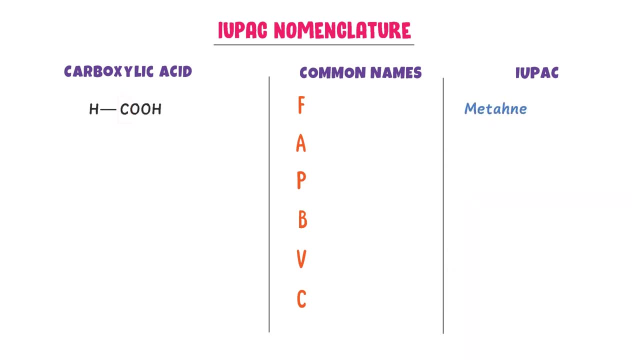 This is only one carbon, I write methane. Remember that for COOH we write COOH. Here we eliminate this E from methane. For this COH, we write OIC. Hence we get methanoic acid. What about its common name? Well, F stands for formic acid, So its IUPAC name. 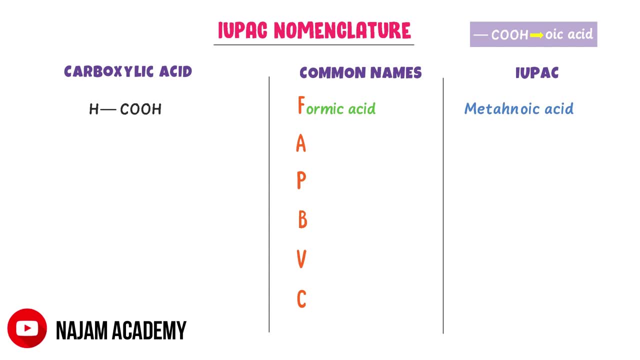 is methanoic acid and its common name is formic acid. Secondly, consider this organic compound. There are two carbons present in this compound. One is carbonic acid and the other is methanoic acid. So this carbonic acid is methanoic acid and this carbonic acid is methanoic acid. 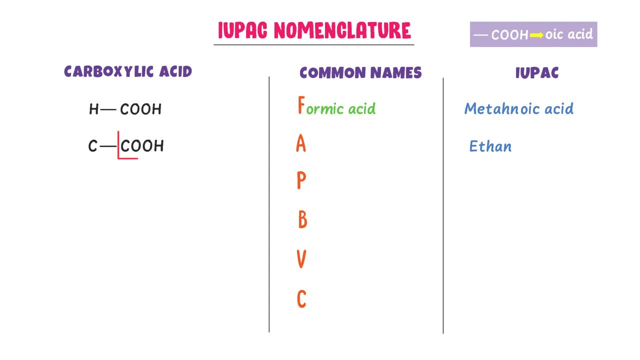 There are two carbons present in it. I write ethane For COOH, I write OIC acid, So I get ethanoic acid. What about its common name? Well, A stands for acetic acid, So the IUPAC. 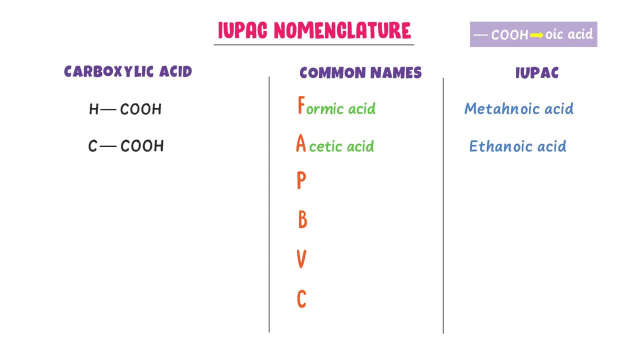 name of this compound is ethanoic acid and its common name is acetic acid. Thirdly, consider this organic compound. There are three carbons present in it. I write ethanoic acid. So there are four carbons present in it. I write butane For COOH, I write propionic. 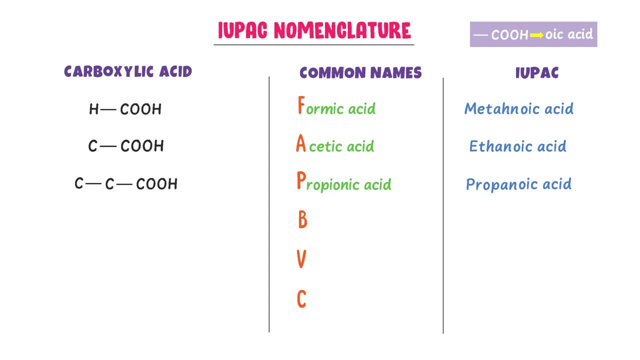 acid. What about its common name? Well, C is propionic acid, So cartobas B minus 1, it's propionic acid. I write propene. images above, pictures below. I write oic acid, I get butanoic acid. 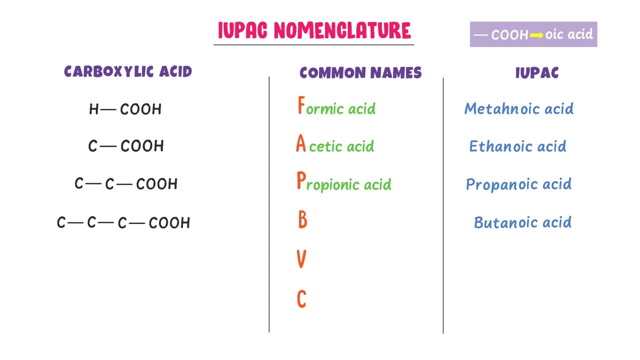 What about its common name? Well, B stands for butyric acid. So the IUPAC name of this organic compound is butanoic acid and its common name is butyric acid. Fifthly, consider this organic compound. There are five carbons present in it. 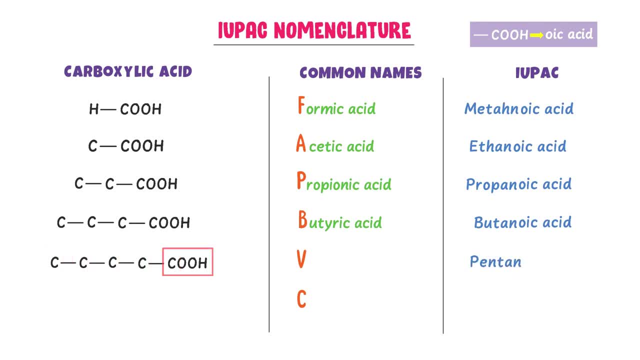 I write pentane For COOH. I write oic acid, I get pentanoic acid. What about its common name? Well, V stands for valoric acid. So the IUPAC name of this compound is pentanoic acid and its common name is valoric acid. 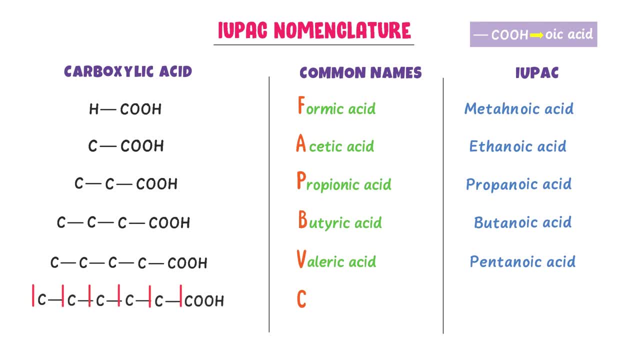 Finally, consider this organic compound. There are six carbons present in it. I write hexane For COOH, I write oic acid, I get hexanoic acid. What about its common name? Well, C stands for caproic acid. 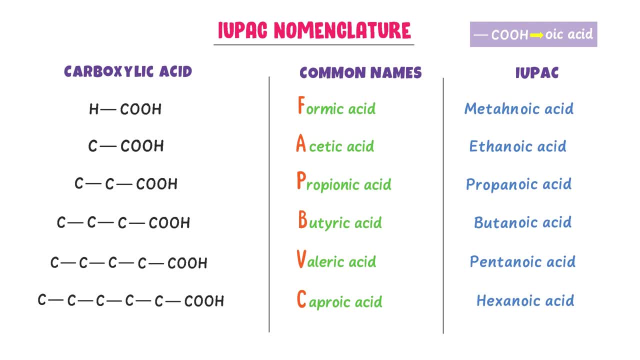 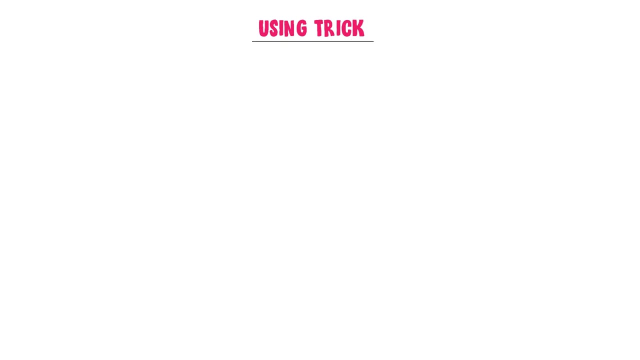 So the IUPAC name of this organic compound is hexanoic acid and its common name is caproic acid. Thus, by this way, we can easily name carboxylic acids. Now let me teach you that how quickly we can use this trick in any exam. 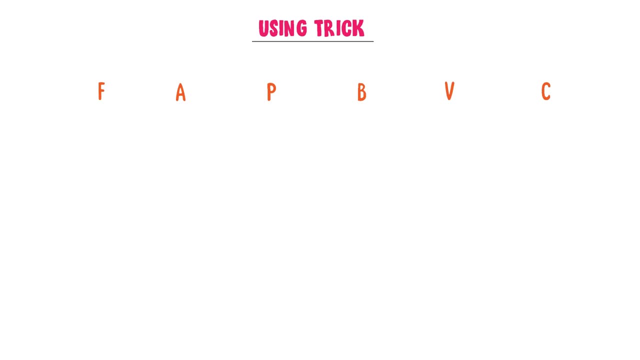 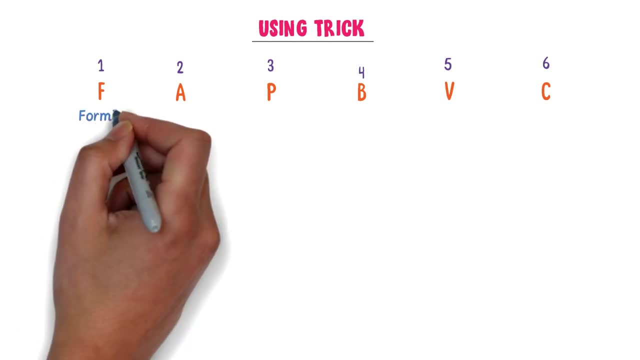 If there is one carbon in carboxylic acid, it is formic acid. If there are two carbons, it is acetic acid. If there are three carbons, it is propionic acid. If there are four carbons, it is butyric acid. If there are five carbons, it is valoric acid. If there are six carbons, it is caproic acid. Thus, this is the most easy trick to remember the common names of carboxylic acids. Hence noted down this important trick. 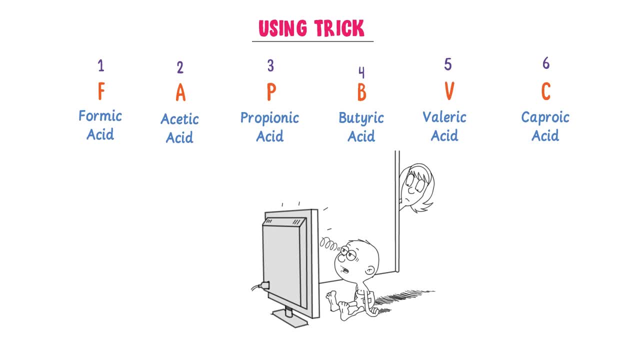 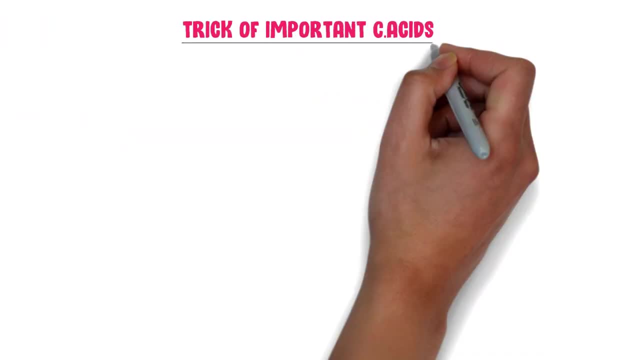 Also, let me teach you some important carboxylic acids whose IUPAC names and common names are asked in exam. My personal mnemonic or trick is to write: Oh, my son go away. Let me repeat it, Oh, my son go away. And I write 2,, 3,, 4,, 5, 6.. 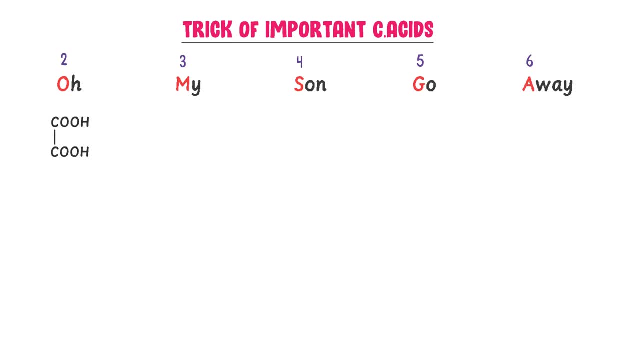 Now consider this organic compound. There are two carbons present in it. I write ethane. Also, there are two carboxyl groups. I write dioic acid. I get ethandioic acid. What about its common name? Well, O stands for oxalic acid. 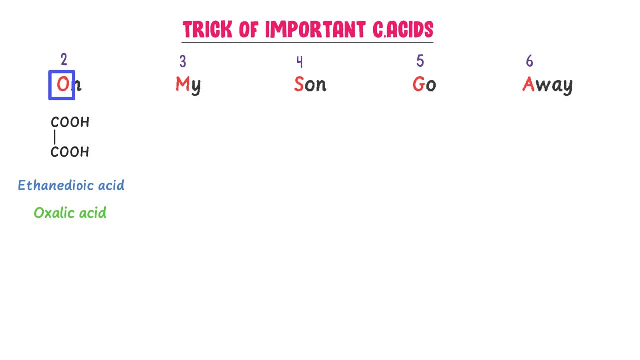 So the IUPAC name of this compound is ethan-dioic acid And its common name is oxalic acid. Secondly, consider this organic compound. There are three carbons present in it. I write propane. The carboxylic groups are present at first and third position. 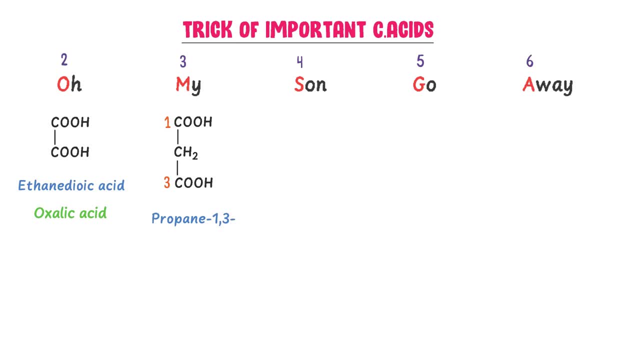 I write 1, 3.. For these two COOHs, I write dioic acid. I get propane 1, 3.. Dioic acid acid. What about its common name? Well, M stands for malonic acid. So this is the IUPAC. 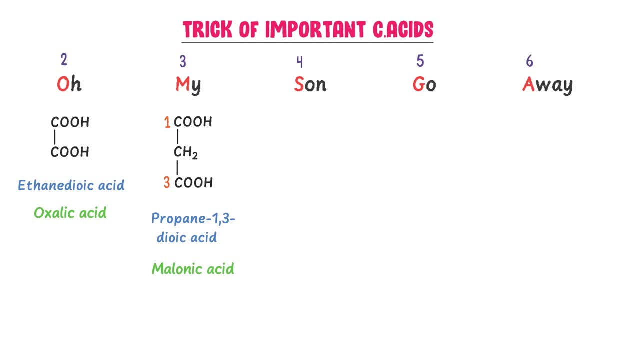 name, and this is the common name of this organic compound. Thirdly, consider this organic compound. Remember that this too means 2 times CH2.. There are 4 carbons present in it. I write butane. The carboxyl groups are present at 1st and 4th position. I write 1,4.. For these, 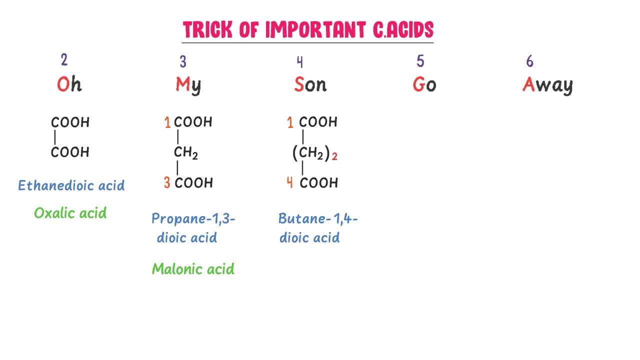 2 COH. I write dioic acid, I get butane 1,4-dioic acid. What about its common name? Well, S stands for succinic acid, So this is its IUPAC name and this is its common name. Fourth, 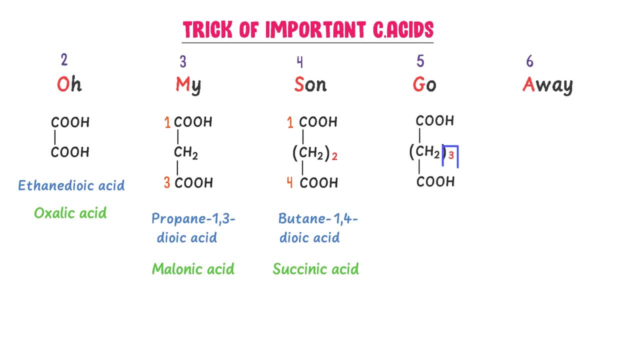 ly. consider this organic compound. This 3 means 3 times CH2.. There are 5 carbons present in it. I write pentane. The carboxylic groups are present at 1st and 5th position. I write. 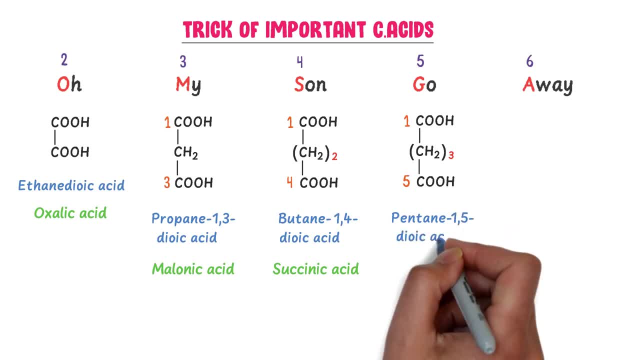 1,5. And then I write dioic acid. I get pentane 1,5-dioic acid. What about its common name? Well, G stands for glutaric acid. So this is its IUPAC name and this is its common name. 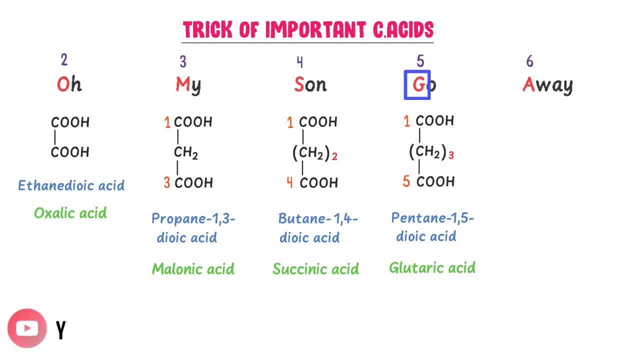 Lastly, consider this organic compound. This 4 means 4 times CH2.. There are 6 carbons present in it. I write hexane. The 2 functional groups are present at 1st and 6th position. I write. 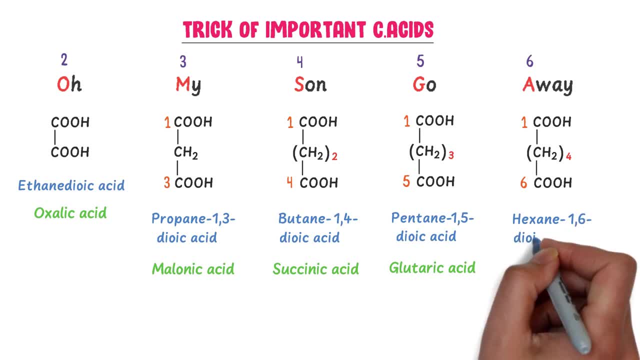 1,6.. Also, I write dioic acid. I get hexane 1,5-dioic acid. What about its common name? Well, A stands for adepic acid. This is its IUPAC name and this is its common name.